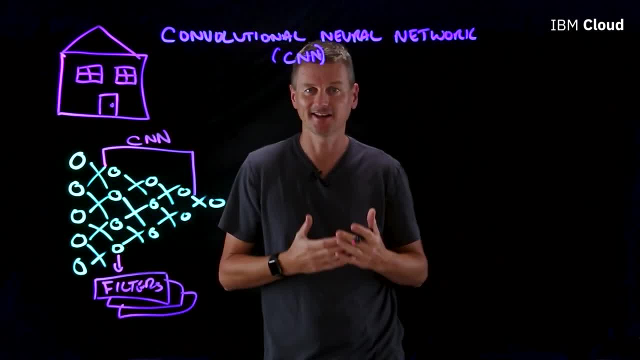 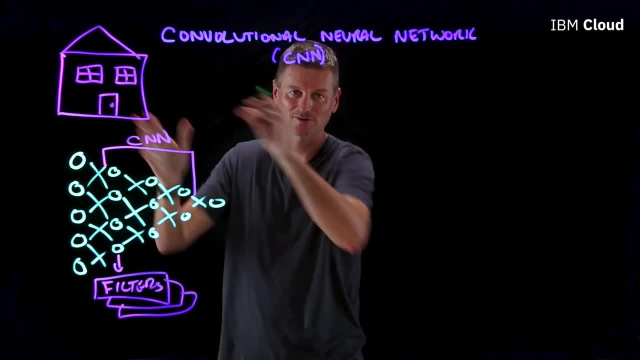 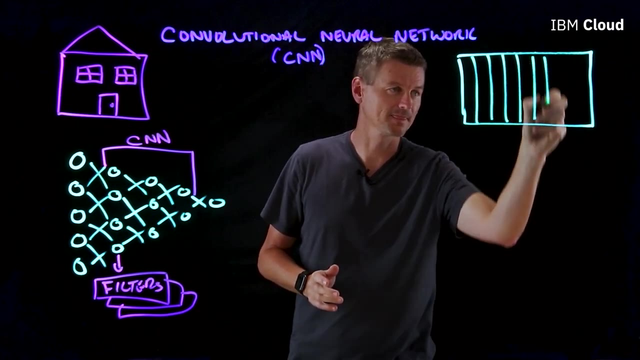 the pattern recognition that CNN is so good at. So let's apply this to our house example. Now, if this house were an actual image, it would be a series of pixels, just like any image. And if we zoom in on a particular part of this house, 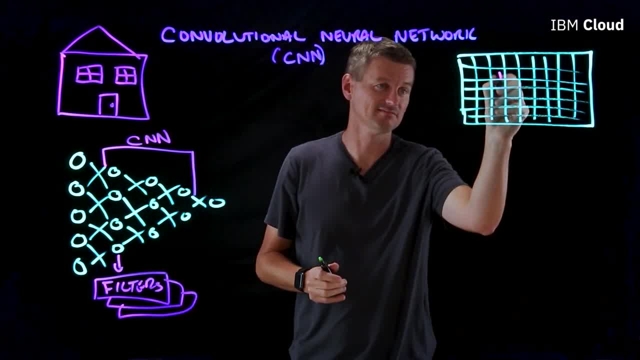 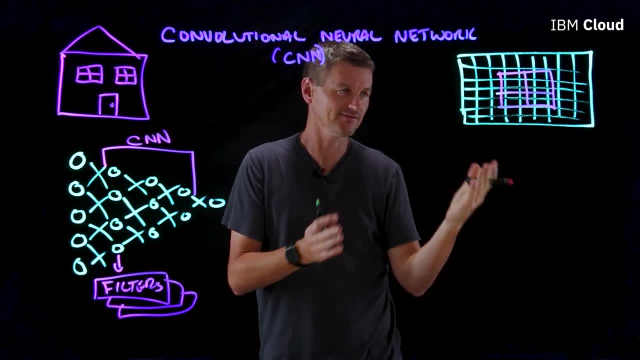 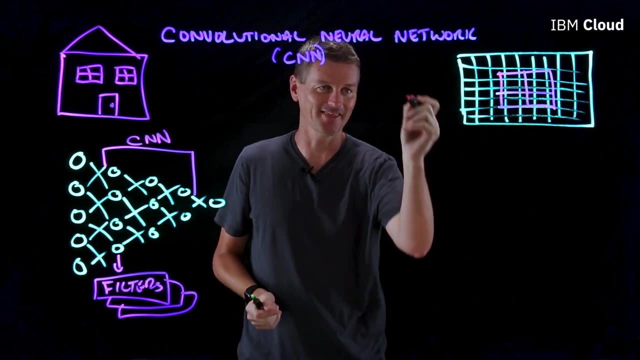 let's say we zoom in around here, then we would get well, the window. And what we're saying here is that a window consists of some perfectly straight lines, Almost perfectly straight lines, But you know, a window doesn't need to look like that. 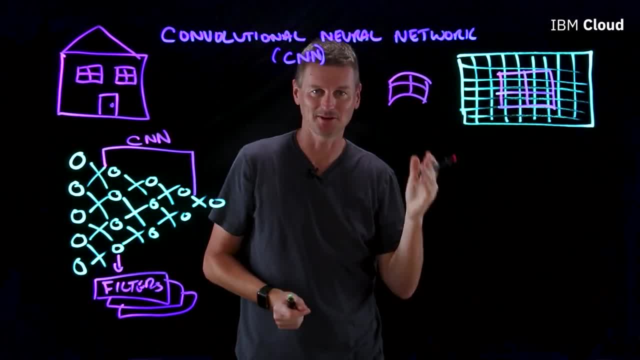 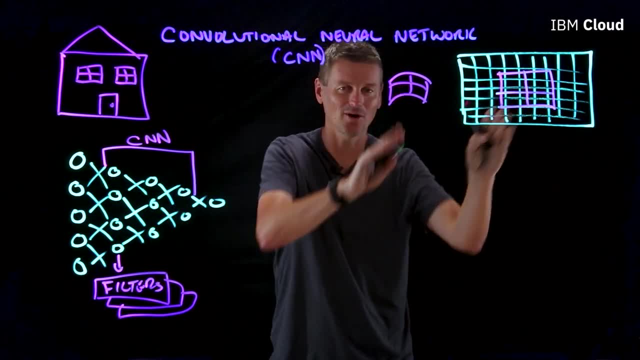 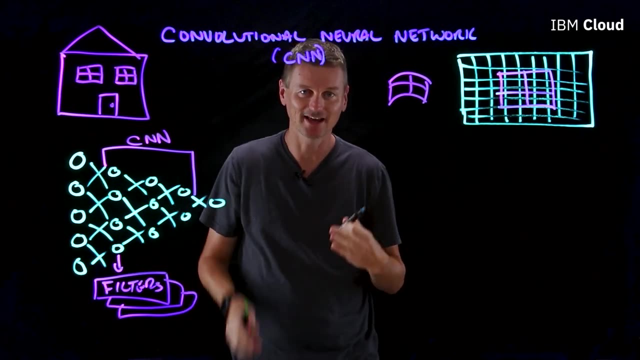 A window could equally look like this, and we would still say it was a window. The cool thing about CNN is that, using filters, CNN could also say that these two objects represent the same thing. The way they do that, then, is through the application of these filters, so let's take a look at how that works. 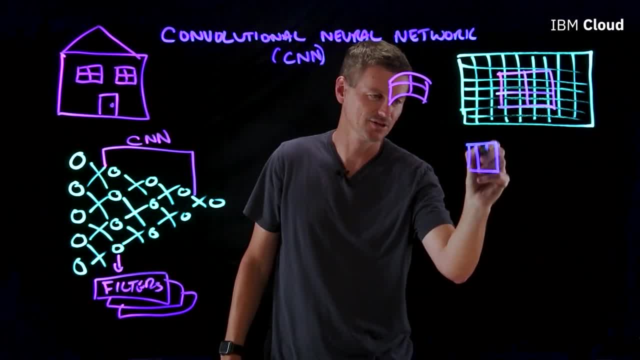 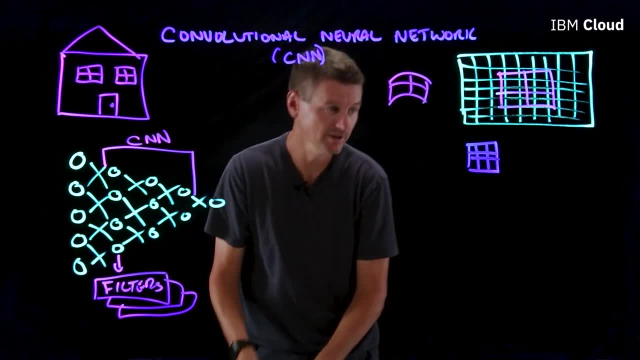 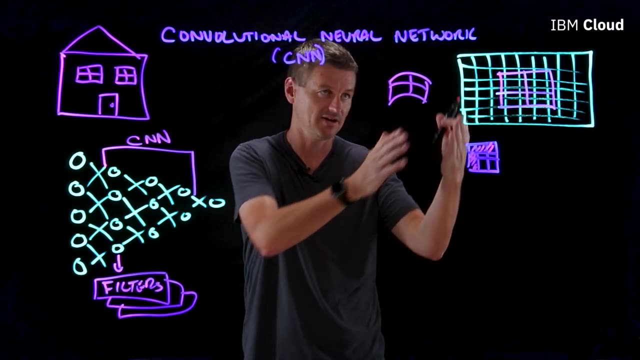 Now, a filter is basically just a three-by-three block And within that block we can specify a pattern to look for. So we could say: let's look for a pattern like this, a right angle in our image. So what we do is we take this filter. 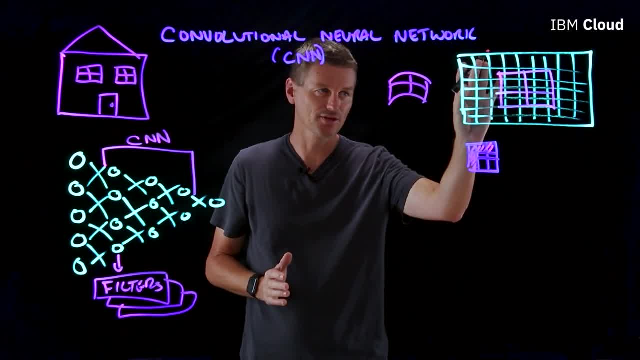 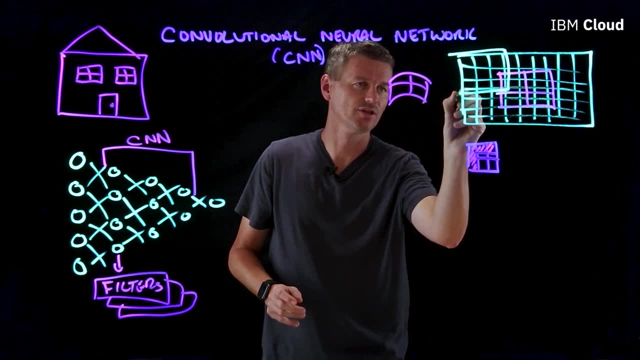 and it's a three-by-three block here. We will analyze the equivalent three-by-three block up here as well. So we'll look at first of all these, this first group of three-by-three pixels, and we will see how close are they to the filter shape. 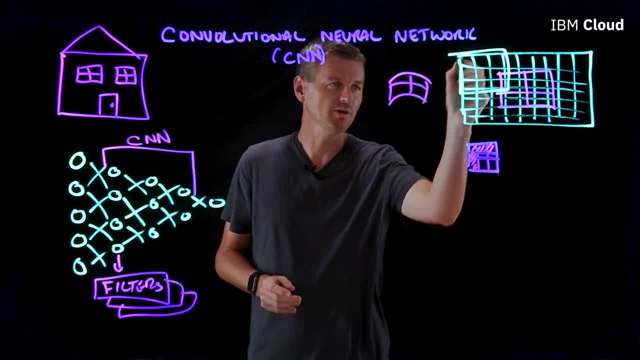 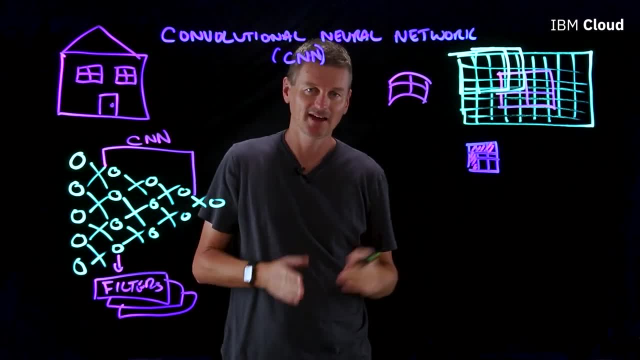 And we'll give that a numeric score. Then we will move across one column to the right and look at the next three-by-three block of pixels and score how close they are to the filter shape And we will continue to slide over or convolt. 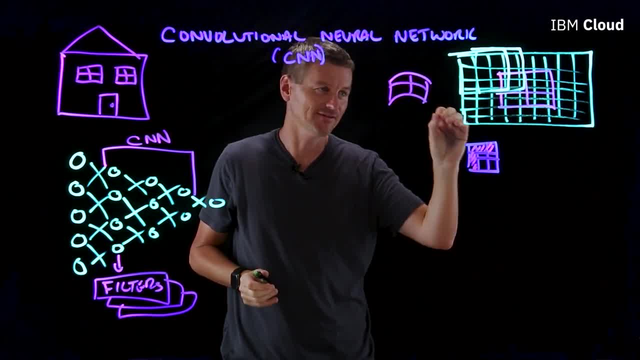 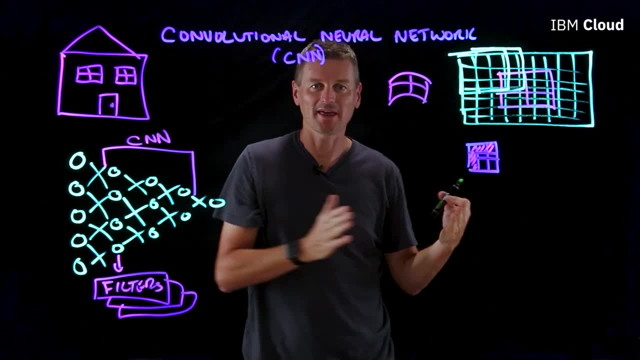 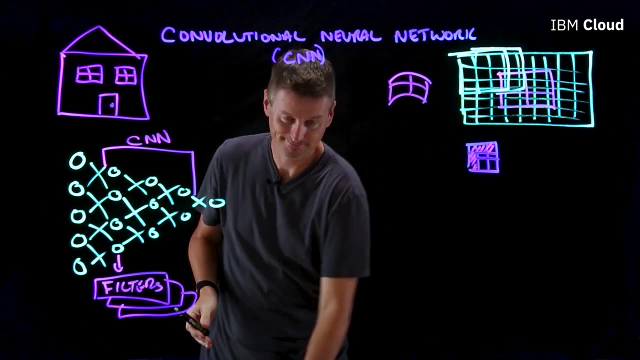 over all of these pixel layers until we have mapped every three-by-three block. Now, that's just for one filter, but what that will give us is an array of numbers that say how closely an image matches our filter. But we can add more filters. 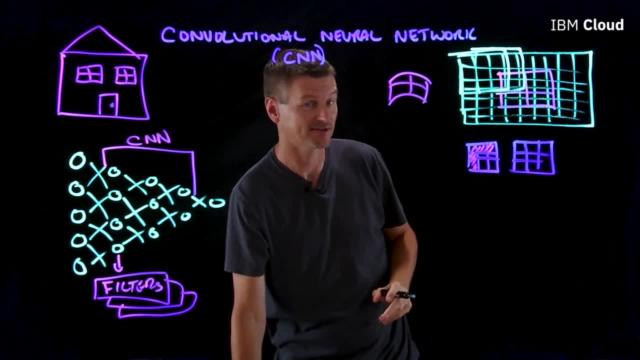 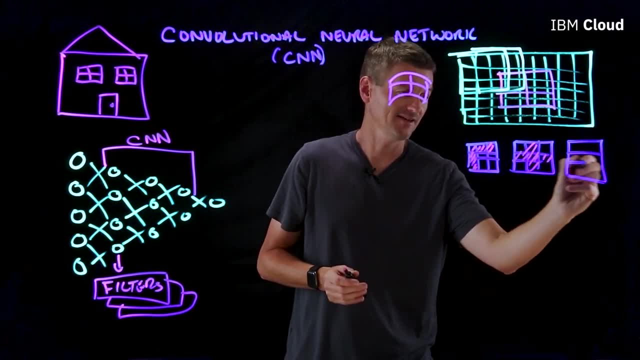 So we could add another three-by-three filter here, and perhaps this one looks for a shape like this. And we could add a third filter here, and perhaps this looks for a different kind of right angle shape If we take the three-by-three block.